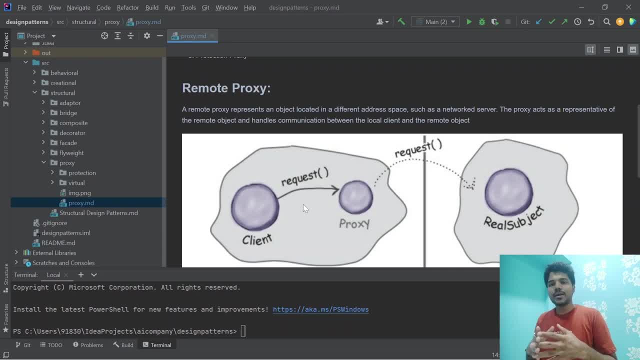 which is there, which is there over the network, so we- so client is not basically direct, directly requesting to the real object. so if you have a proxy in our address space now, client request will go to the proxy and proxy will basically request to the real object and then the request. 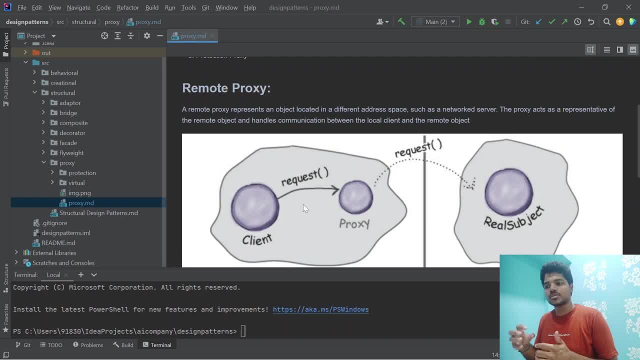 whatever response comes comes from the real object right it will stores in the proxy for the next client to serve. so here proxy will act, will basically acting as a middle person between the client and the real object. so a remote proxy represent an object located in different address space, such as a network server. the proxy acts as a representative. 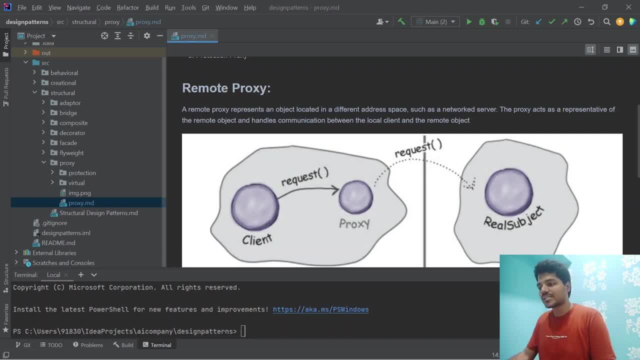 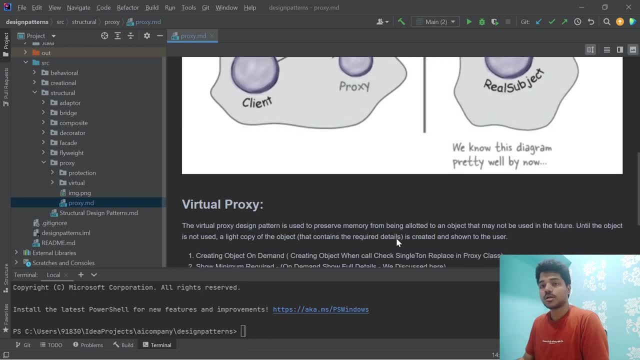 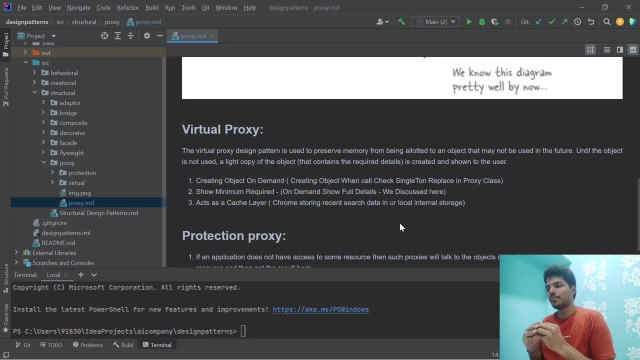 of the remote object and Handel's communication. this is the most important one: Handel's communication between the local client and the remote object. now let's discuss about what is virtual proxy. so virtual proxy is a pattern used to preserve memory from being allocated to an object. let's 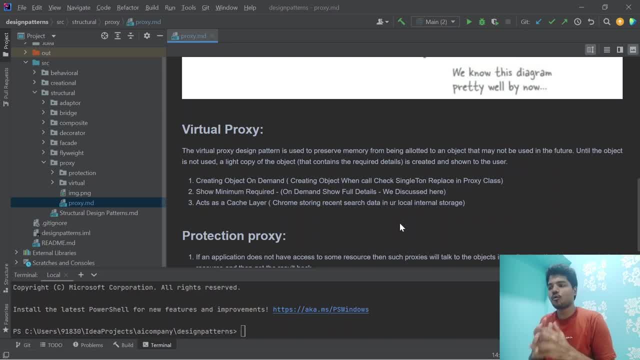 say, before going into a complete definition, right, let's have this thing: what is preserving memory? which means like there is a real object which is basically taking like a huge amount of memory during response, like while returning the response to the user. which means like that huge amount of object is basically loading at the client side. 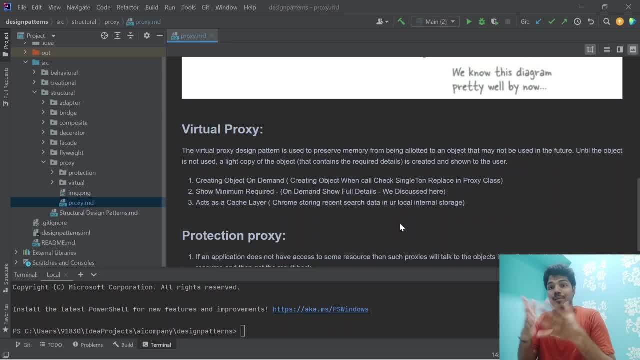 So sometimes it is not necessary for the client to see the complete object like. if client is seeing complete object, it may not be responsiveness, depending upon the client. bandwidth to the internet or like client response time might be increases because it should load the complete object right. 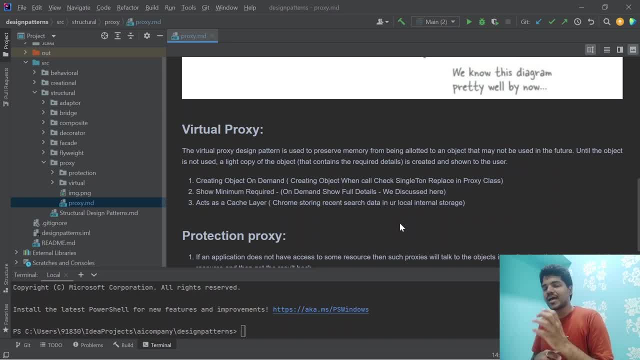 So, which means that virtual proxy is basically acting as a lightweight to the original object, which is basically heavy memory intensive object like So virtual. let's see the complete definition, you will understand more. So virtual proxy design pattern is used to preserve memory from being allocated to an 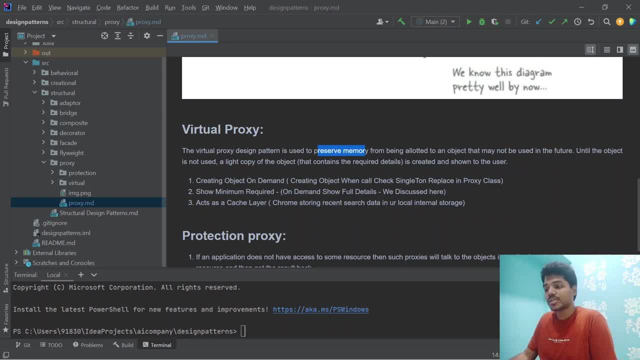 object that may not be used in the future, like until the object is not used, a light copy of the object is created, Which means if someone exclusively wants to use the object, then the object is not used in the future. If someone wants to access the original object, then only the original object will be provided. 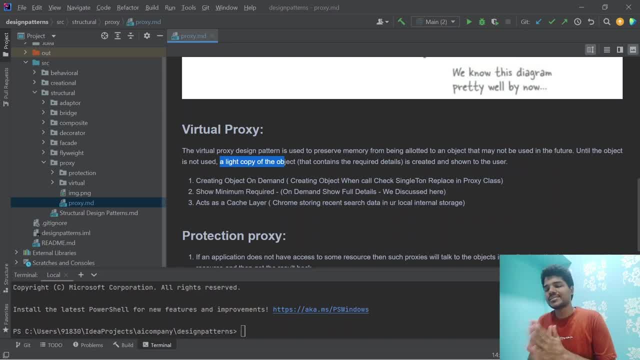 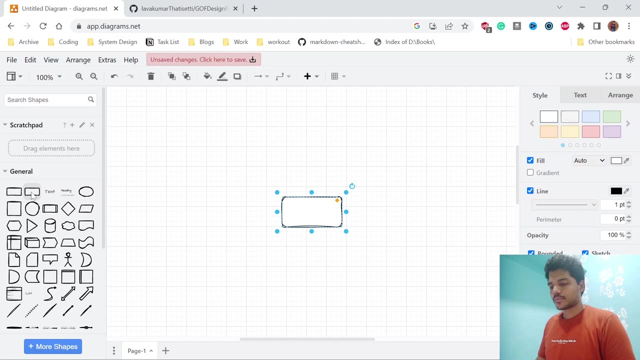 if not only light object will be shown like. So that's exactly what is virtual proxy like. now let's discuss virtual proxy through examples so that you get better idea about what exactly virtual proxy. Let's take about example of like, let's say Amazon, like. and also, for now, let's take about 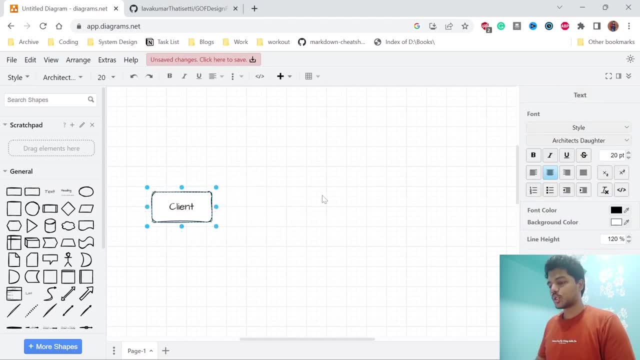 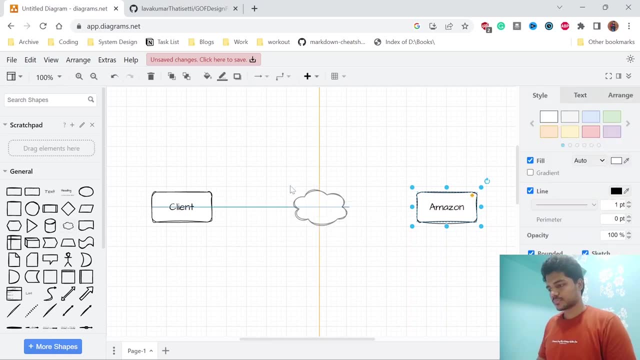 Amazon. So we have a client. So client is trying to access a resources Like these are like Amazon resources over the cloud. So this is a setup, right. So client basically tries to access the Amazon resources over the cloud. So there are like multiple images presented in the Amazon website like: so let's say it. 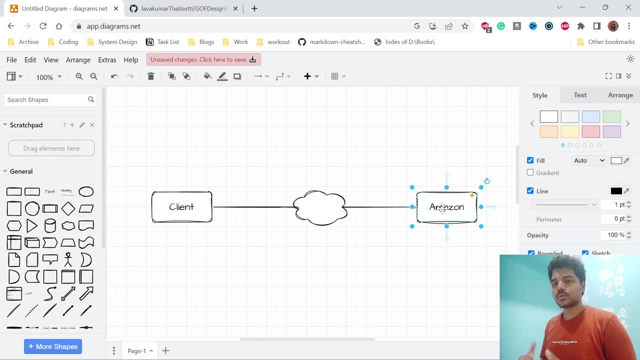 can be. it can be through serving through CDNs or it can be serving through any like what? whatever options Amazon have. But let's say client wants to see the images like. So, for example, there might be some high resolution images and there might be some low resolution. 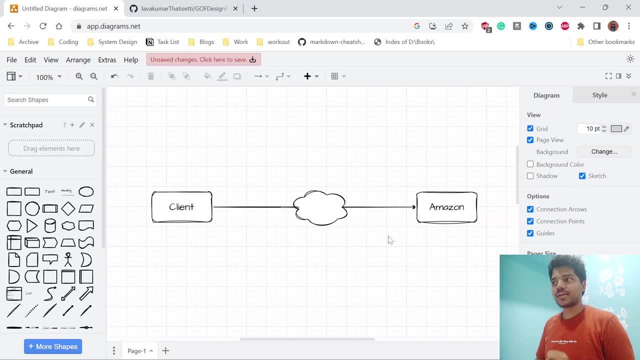 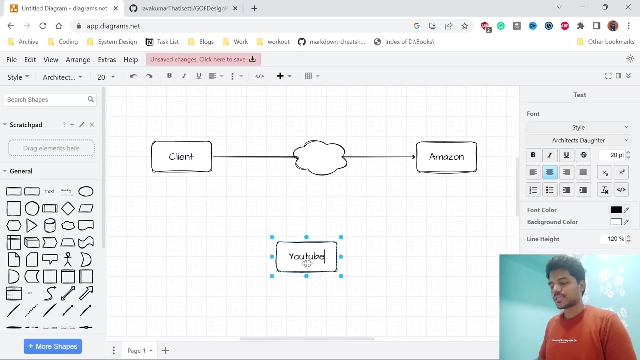 images, If you, the best example we can see. it is like Netflix. if you watch the videos on Netflix, right there is like whenever someone uploads the video on Netflix or YouTube, in the sense: So what? what exactly happened when someone- let's say, we have a YouTube- someone tries? 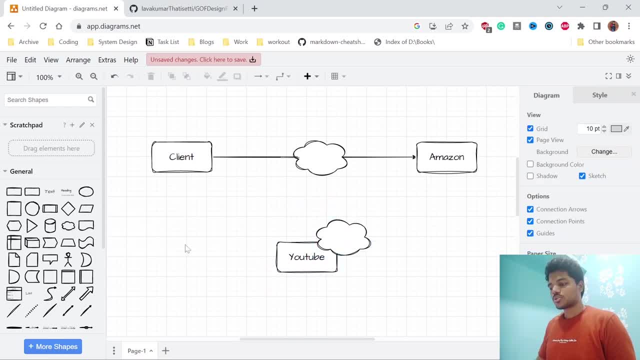 to upload something like onto YouTube. So what exactly will happen? So YouTube will basically, First of all, YouTube will divide those videos into multiple chunks and from the multiple chunks, each chunks, they will, they will. YouTube basically creates multiple videos again. So this chunk, let's say one video, are divided into six different chunks. 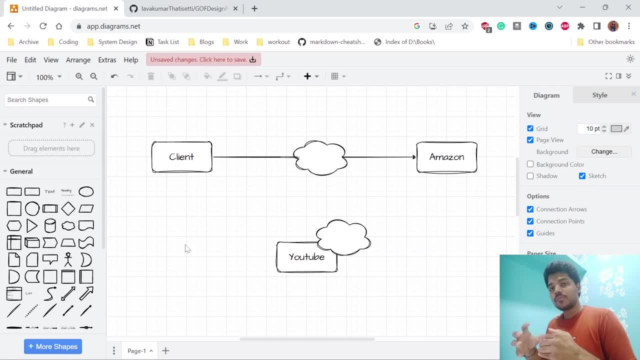 So each chunk. again it will divide it into like let's say five. So it means resolution is like, let's say one kind. one image can be like, let's say, 720 pixel image. One image can be 4K, one image can be 1080. 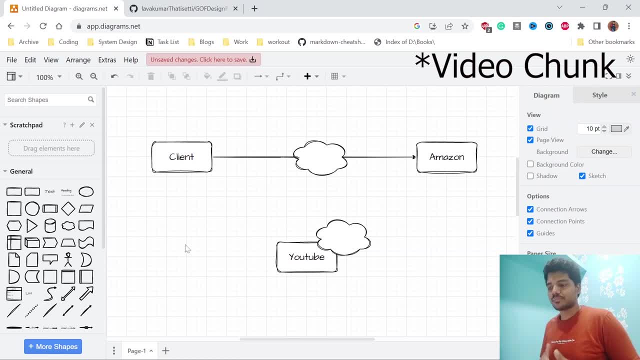 One image can be 4K. One image can be 4K. One image can be like 240, something which means what- and also, yeah, further encoding will be happen, like multiple formats, also MP4, or like to support Mac OS, all those things, but that is not what we are discussing here. 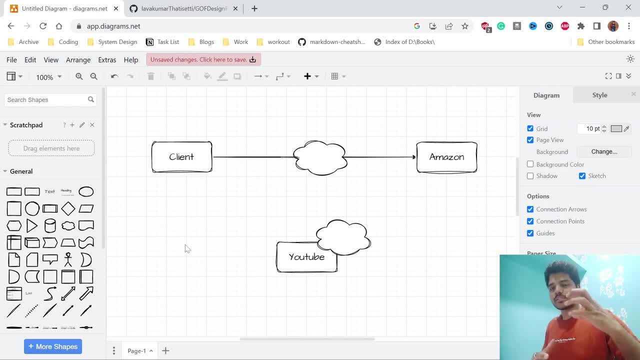 The main goal is like one single video, and that too, only one chunk, is basically dividing into multiple resolution videos, which means, let's say, I, let's say when I was streaming the YouTube, when I was watching the YouTube video, right, Which means There is a possibility that I cannot get the original object, which is basically 4K object. 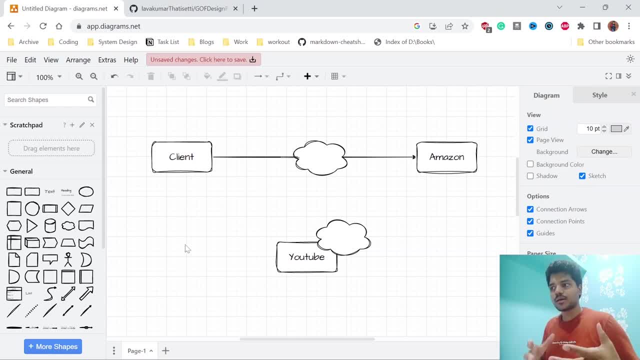 It might, it might not be possible whatever. whatever the person uploads the video, I may not be see the exact pixel video. I mean I may see that 480 or 240. it will adjusted by YouTube automatically depending upon the my bandwidth, which means those are like basically proxies of to the original object. 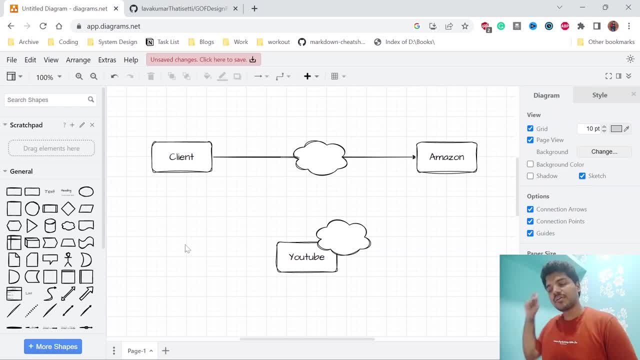 So whenever I, whenever I requested for the original object- which means I requested for the original object, Which means I, I did- I want to see the 4K. whenever I selected that button in the settings tab right, then only the original object will be loaded like. otherwise it won't be load like. 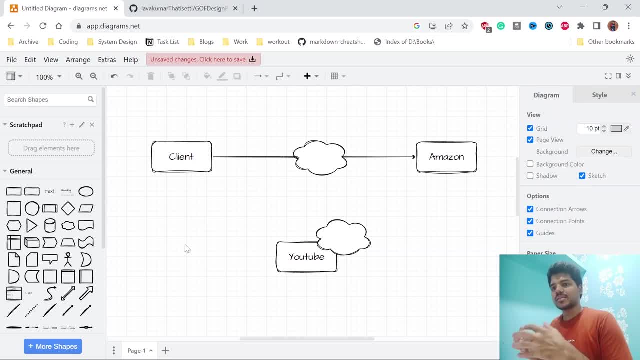 so it will only serve through proxy objects, which basically call it low resolution objects, like. so that is the one best example of how images or video comparison basically working and also serving to the users. So that is one example. Let's take one more example. 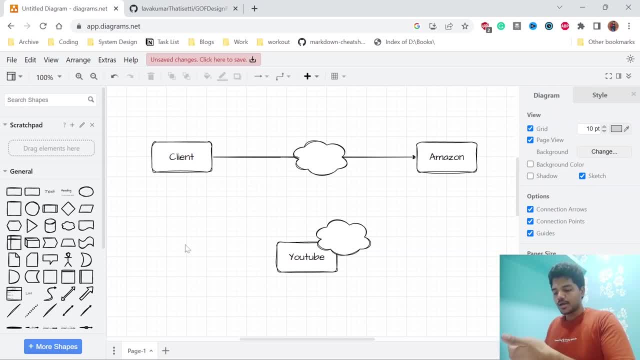 So You're basically viewing Video, Amazon reviews: So someone basically reviewed, someone basically reviewed something on Amazon. So you're you're viewing the reviews and ratings, everything. So if you observe something, if you watch, if you watch through, if you watch on mobile and 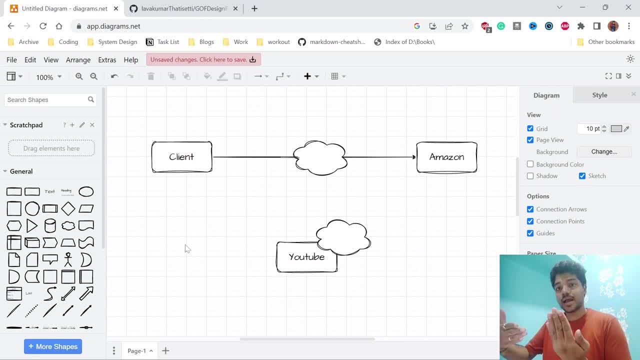 if you watch on like desktop, there is a different kind of variables will be presented. Let's say, if you're watching desktop, right, you will see full content, you will see rating, you will see image, everything. when you're watching on desktop like or desktop or video. 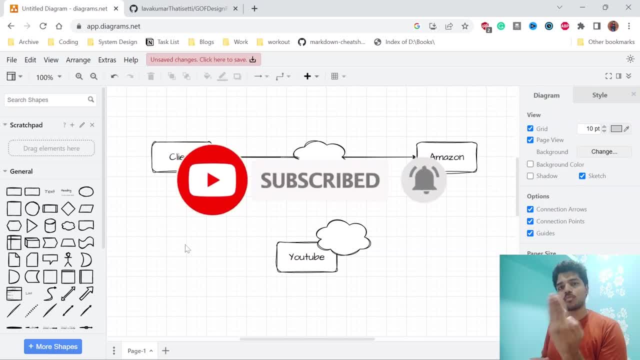 but when you're watching on mobile- with mobile is very small, right like so- which means you can only see the ratings and only one liner of the, let's say, description- you won't see anything. if you want to see, you need to go there and you're externally asking the Amazon. 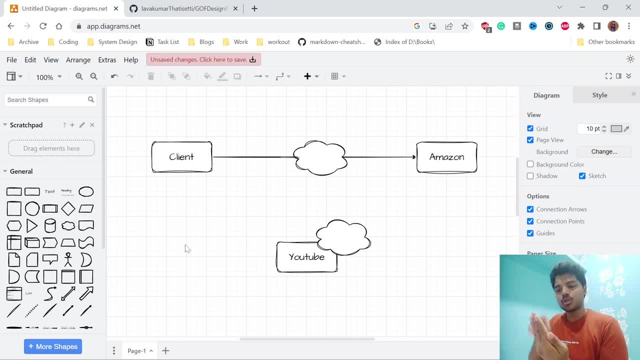 to provide the original object. So in the mobile you're seeing only the proxy object, not the original object. like whenever you ask the Amazon, it will provide the original object if you want to see the complete detail of the review. So these are the things. 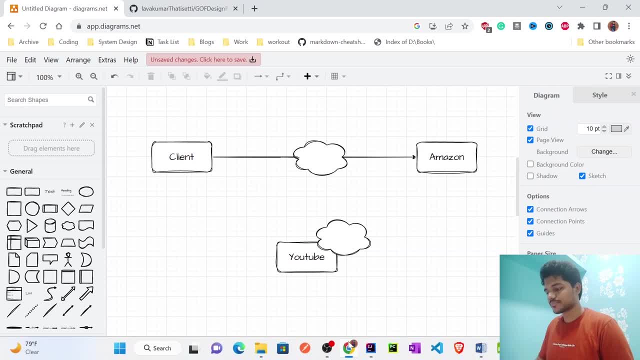 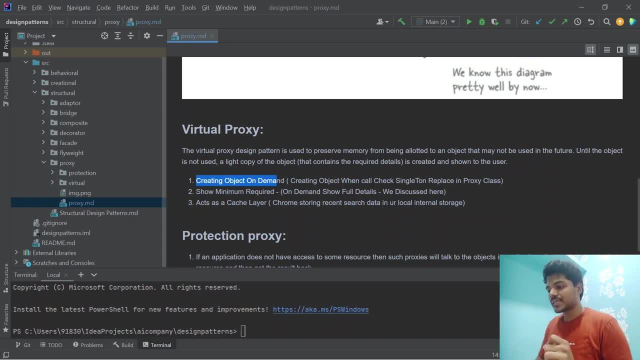 So these will basically categorize as a virtual proxies- now see the definition. So creating objects on demand like basically the main. the main idea of virtual proxies like to preserve memory from being allocated to an object. It can be either through image video compression, it can be either through, like what we are. 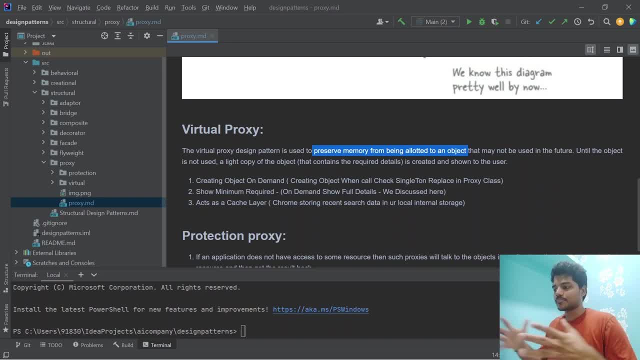 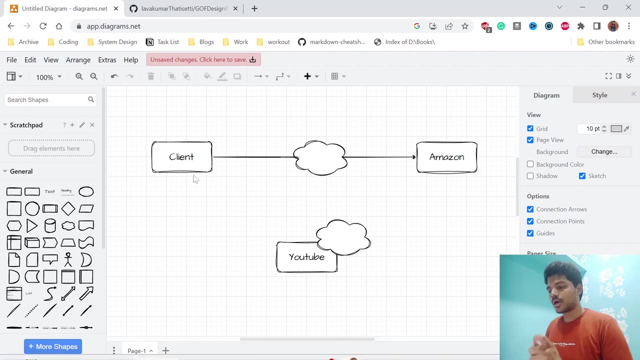 viewing in the multiple resolution, multiple screens. So and also so minimum required. Let's say an Amazon use case And creating an object on demand, let's say YouTube use case, So acts as a cache layer, let's say so. let's say, client, you're accessing something from. 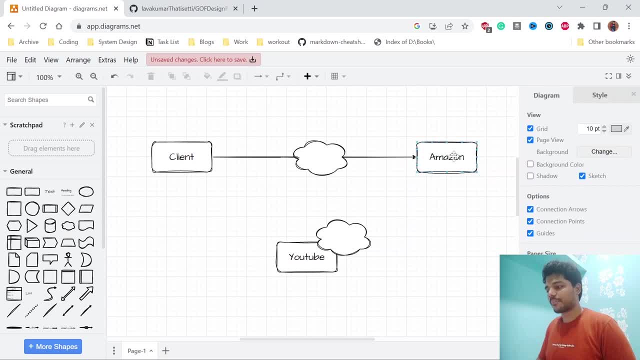 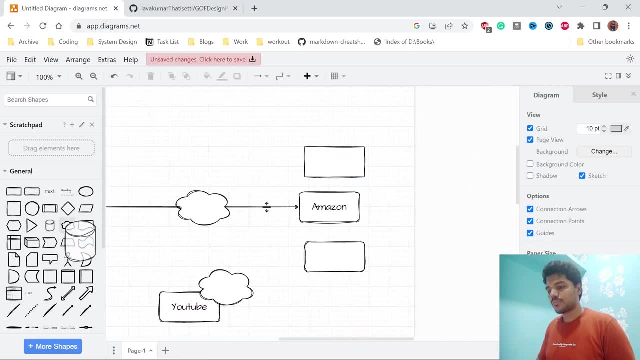 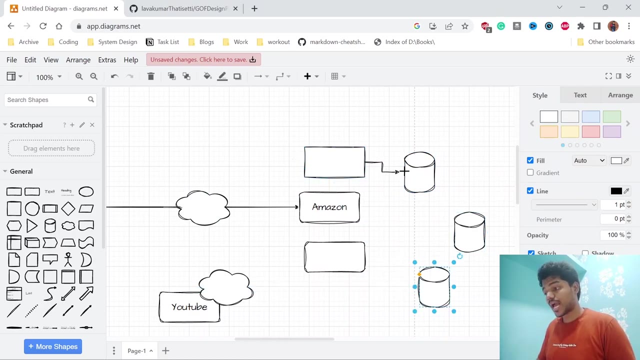 Amazon, which means like Amazon has like multiple services. right, Amazon is not a single service, So Amazon has like n number of services. So and simultaneously, Amazon will basically talk to db's also like multiple db's, which means there are not- there are lot of network calls are being happening, like every every. 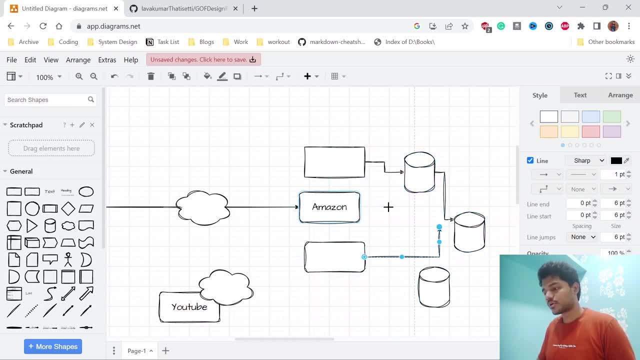 request you made, there are like n number of network calls happening, So these are all like located in the inside the cloud, right? whereas, let's say, when you try to access a request first, it will check whether resource- whatever customer is trying- is present inside the memory or not, which means something like caching- it will check. 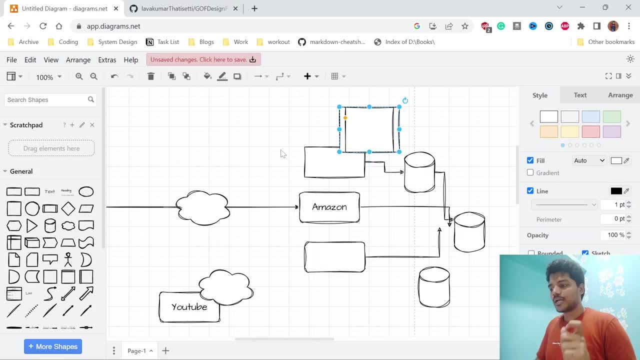 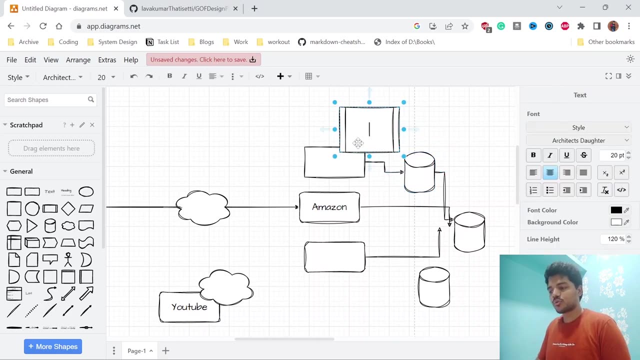 okay, whatever customer is asking is present, it will check whatever customer is asking is presented inside the cache or not. Which means So we are maintaining a cache and also what you call tables in sync. So if something is presented in the cache, So we straight away replying to the customer. hey, customer, this is your whatever requested. 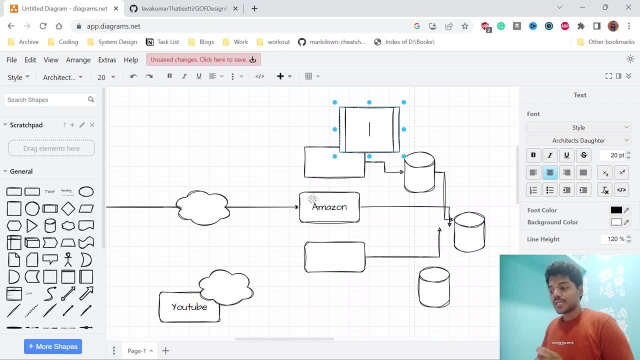 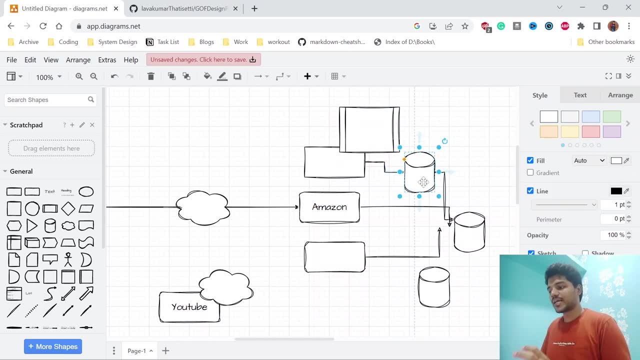 this is your response? If it is not, which means here we are preserving the extra network call, because this- this tables are like basically sits on disk also, which means like into, basically to the network call and also you need to find the exact data, That data where actually stored in the disk and you need to get the data like, which means 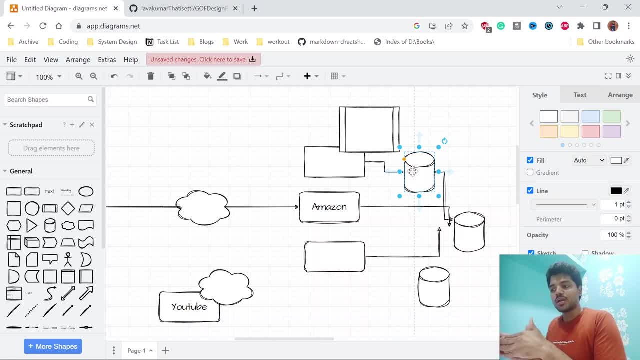 like there is a lot of operations involved. let's say, if you store everything in the cache rate, you will save the lot of seconds- like lot of seconds- as a response time, which is basically improves the user experience. So that's exactly what actually we are saying. and acts as a cache layer. 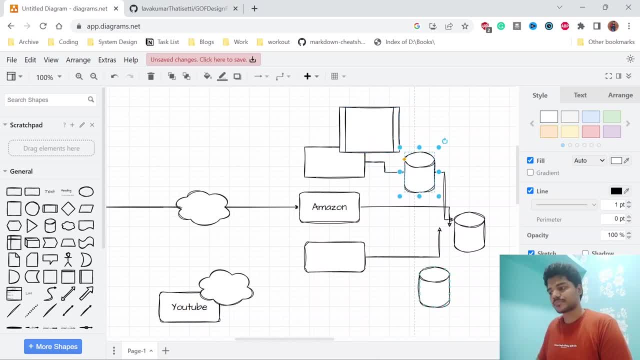 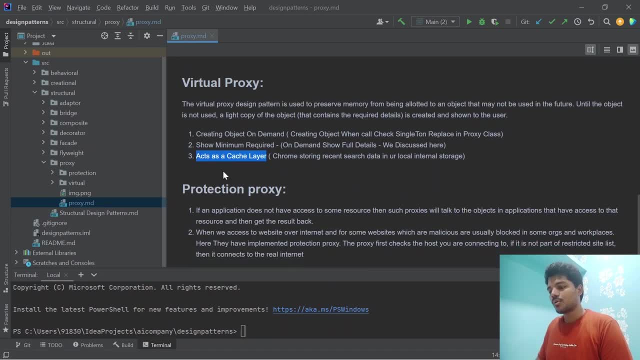 So this is basically categorized as virtual proxy and this is a real object. So I think that's about virtual proxy. we will see that. we will see the examples, like now let's discuss about, like production proxy. Production proxy is like, let's say, you are working in an organization. 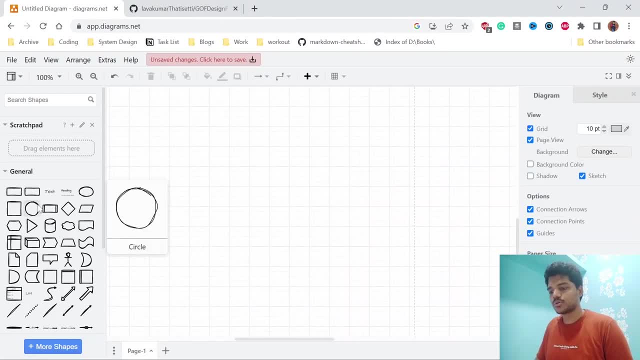 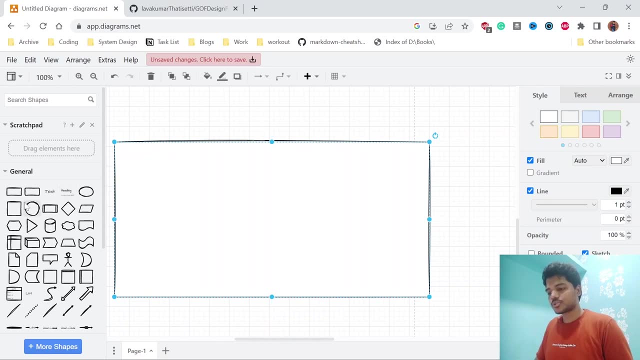 So this also we can illustrate for example, so which you understand better. So let's say you are an organization, So you are working on a company laptop, So this is basically company laptop and your organization basically has some some, basically some restrictions to access the outside internet, like 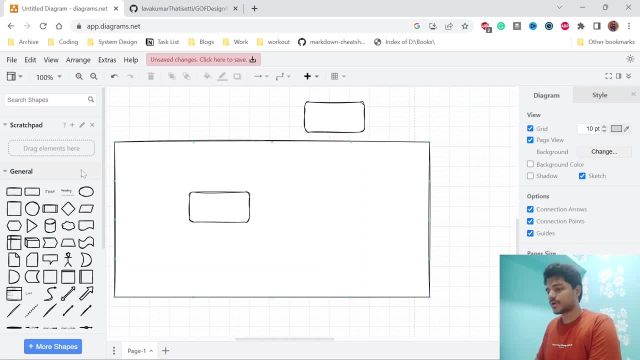 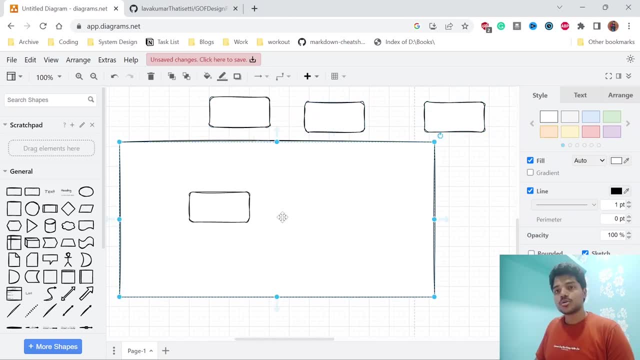 So these are all like, These are all basically different, different outside internet websites. So you need to access all these outside internet websites. So here what exactly will happen? So your company might return some kind of configurations, Okay, whenever a person who are in my network, if it is, if it is trying to access, let's say, 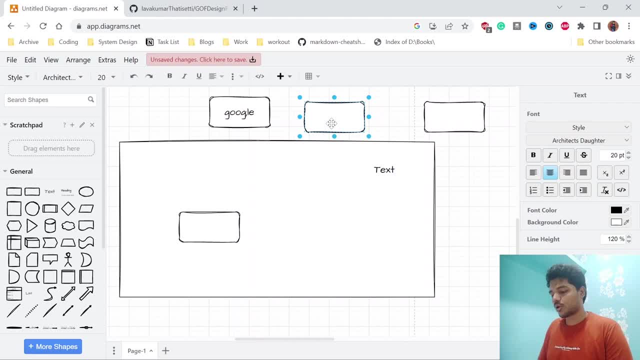 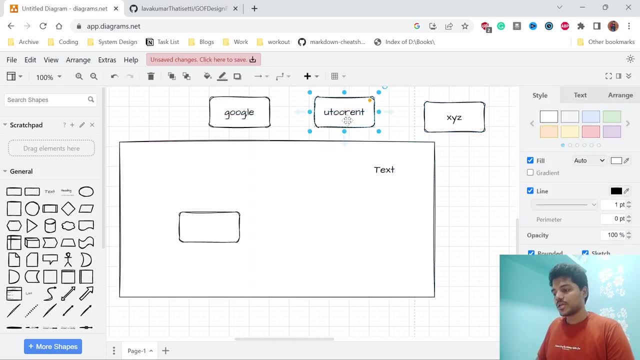 this we can call as like Google, and this we can call as like uTorrent and this we can call as like Google. So this is basically like some xyz website, So which means so there is a restriction at your organization's side, organization's side. 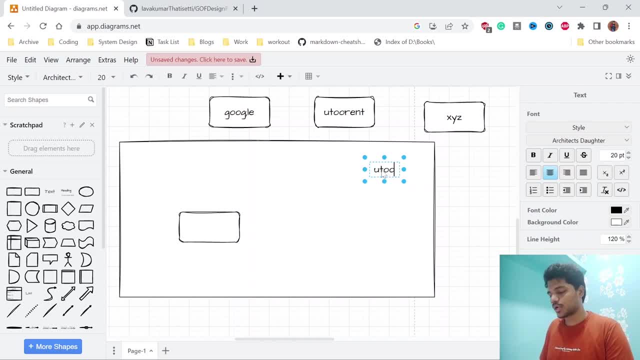 So which means, like so, if someone accessing uTorrent, let me block, like so we are not allowing to access the uTorrent website. So which means, whenever you are trying to request the uTorrent, so every outgoing- basically every outgoing network will be based on the uTorrent website. 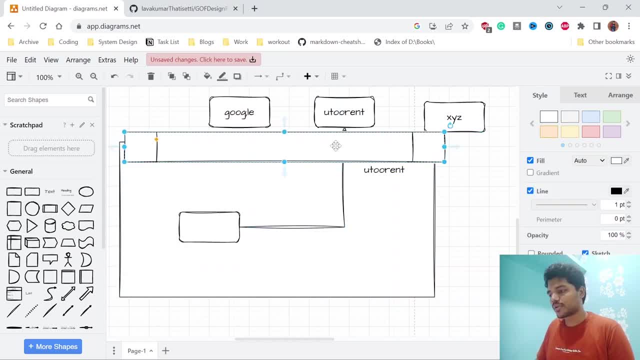 So this is basically what we are doing. So this is basically what we are doing. So this is basically monitored. monitor, basically this. this acts as like a kind of firewall, So every outgoing will be monitored and if you, if it check it first, it will check in. 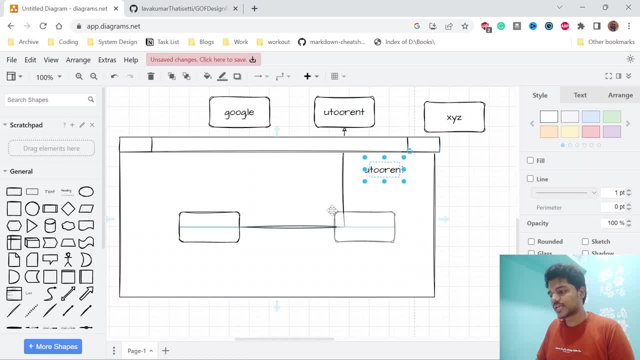 the configuration. Let's say, when you're trying to access first, it will check in the configuration. in this configuration, uTorrent is present. If it is, uTorrent is present, straight away. this request will be rejected. it won't go. but whenever you're trying for Google, then it will check. okay, Google is not there. 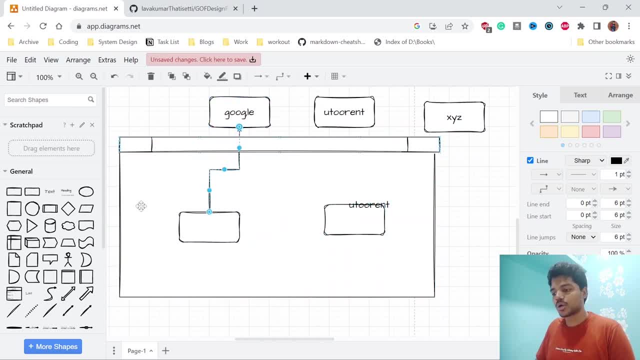 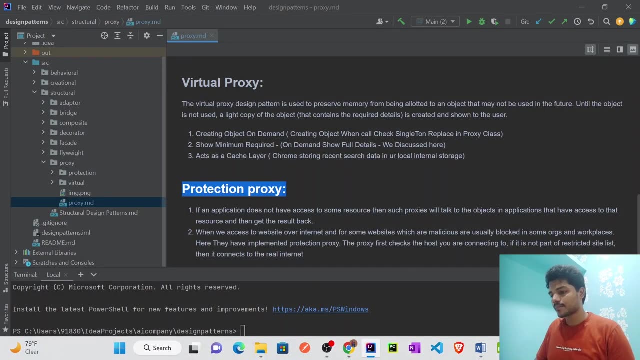 So let's, let's allowing, allowing to request to uTorrent. Okay, So this is exactly protection proxy. you're protecting your network or your organization from malicious content or malicious websites which are presented outside of your network, like. so that's exactly protection proxy. So if an if an application does not have access to some resources, then such proxies will take. 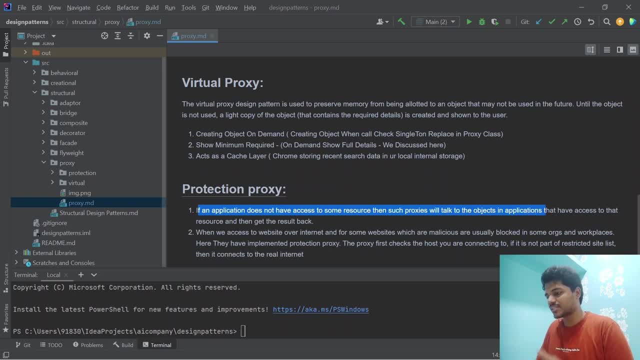 to, to talk to objects in an application that have access to that resource and then get the result back. So when we are accessing over internet, for some websites which are malicious are using in blocked and in some walls and worksplaces, the. so these, these, these we basically call. 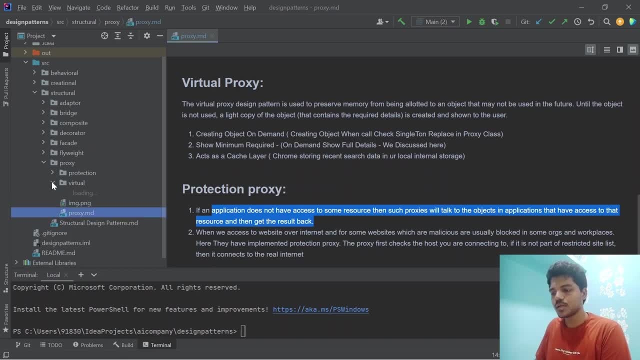 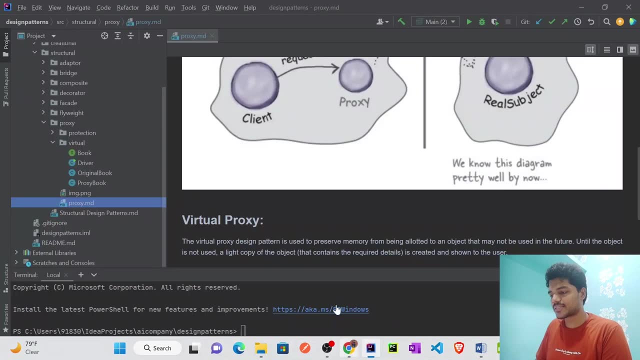 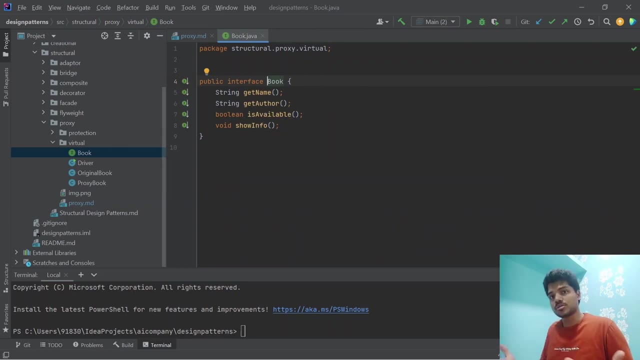 this protection proxy- Let's see the example. All protection proxy and virtual proxy, So video description. So let's see the guidelines, for example, of like Amazon. Like- see the same example. So let's say you have a book here, You're seeing all the books in Amazon. 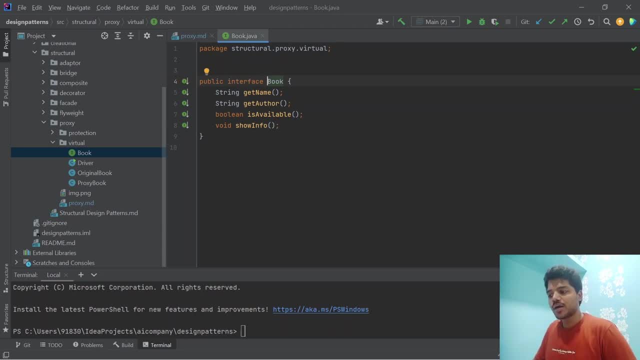 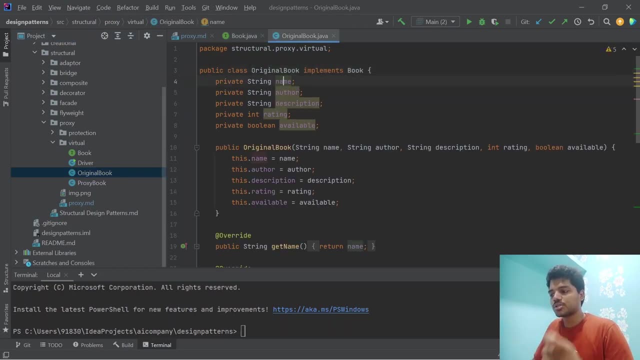 So, which means generally book content, name, author is available in email Also, which is being shown, Info can be description, everything right. So let's see the original book, how the original book which is there in the database look like. So, original book has a name, original book has an author. original book has description. 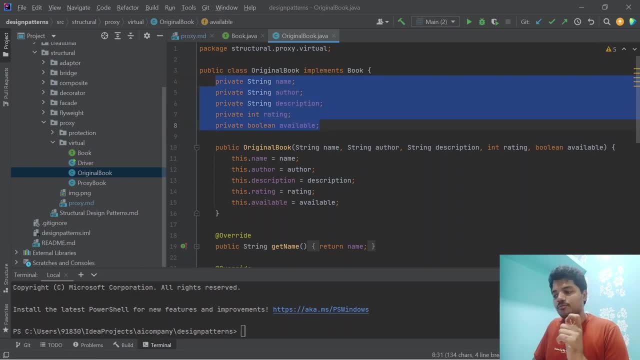 rating available. But if you observe here, what do you think? It's like heavy object, which means if you by mistake, if you include description also in the response, description can be very large, right, So it might not be very responsive when you're viewing description in the mobile. 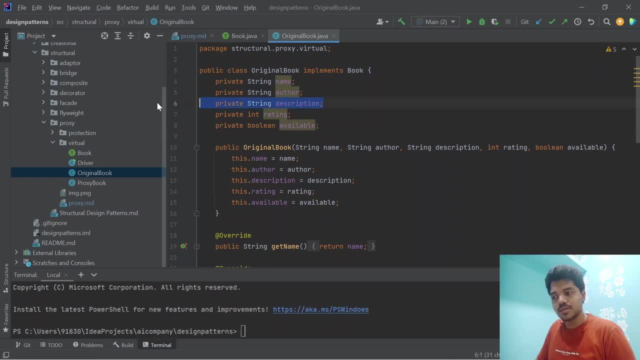 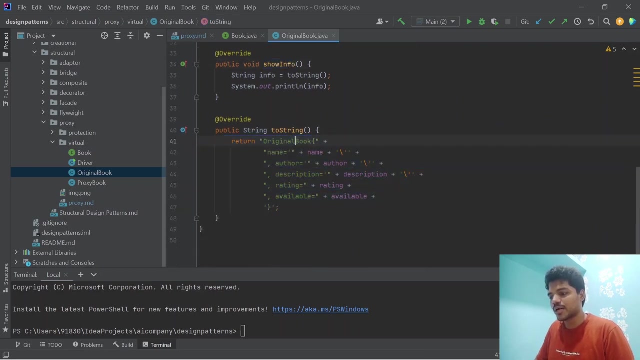 So this is the original book. whenever someone is asking for the original book, you can show, but whenever you're asking generally to see the book, you will hide the description. So in the show info you're basically showing the complete information of the original book. 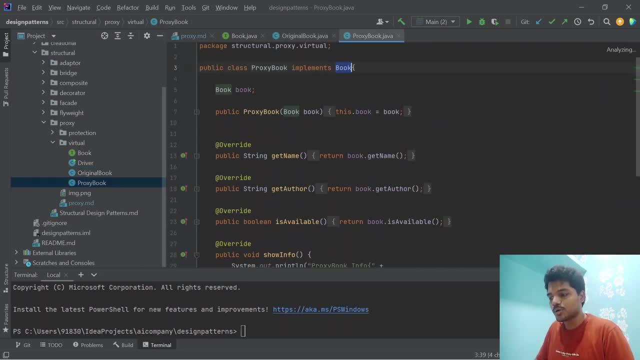 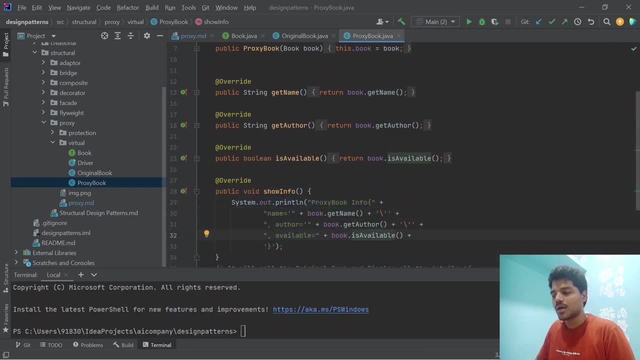 right. Let's say I have a proxy book also which also implements the book. But in the show info I am not showing the description. I'm showing the complete book info. I'm showing only name. author is available or not. 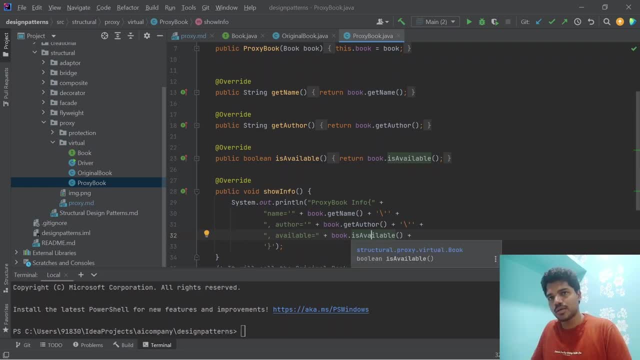 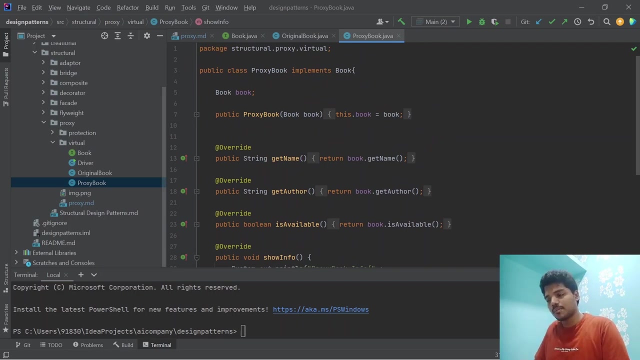 I'm not showing rating. I'm not showing descriptions, anything. I'm not showing anything. I'm just showing only required information. So this can be viewed by any resolution screens. So, but whenever customers wants to access the original book, we're providing a function. 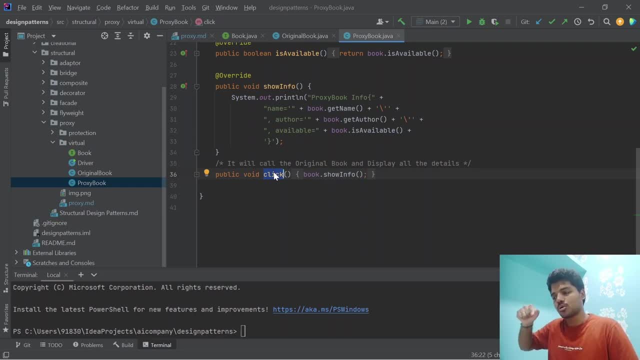 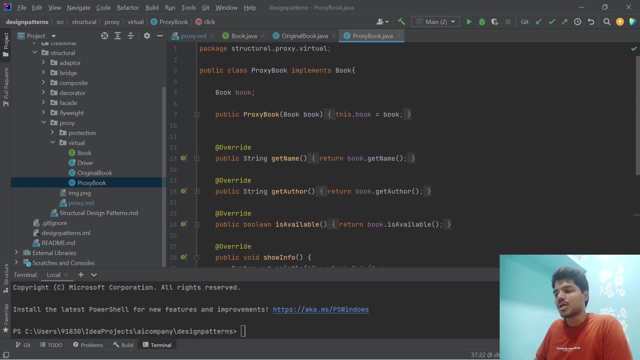 called click functions. If someone is clicking, so he's basically looking for original complete information, complete book information, then we are calling the original book show info method, which means proxy book has like taking a constructor called book, So we need to pass the original book as a constructor to the proxy book. 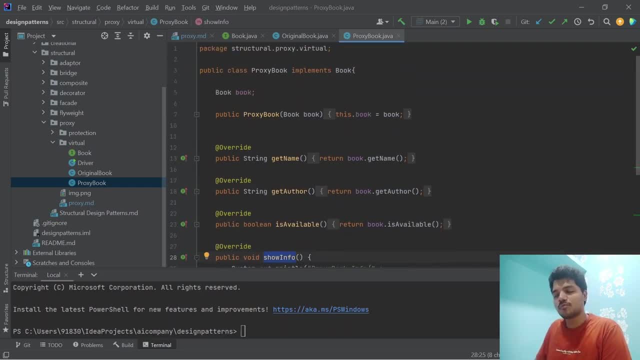 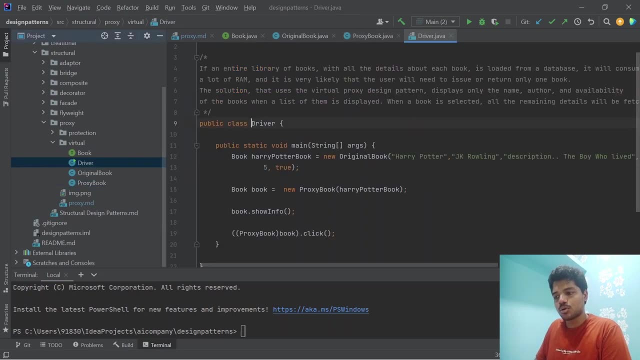 So we'll generally show the show info of the proxy, But someone wants to show the original book. we'll just simply call the proxy bookclick. So let's see the driver code. you'll understand even more better. So here in the driver right. 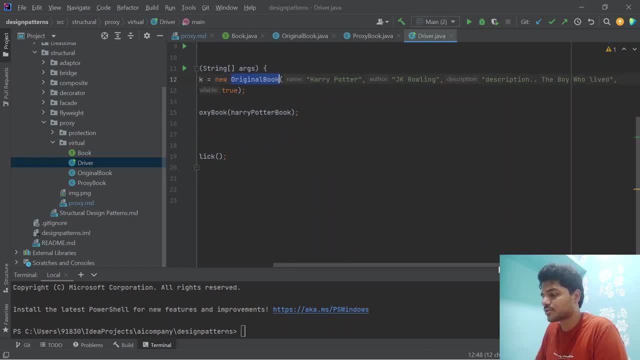 I have an original book. original book has a complete information with- along with description also. So I'm a fan of Harry Potter, So I have included Harry Potter first chapter. So I have a Harry Potter book. So now I am proxying the Harry Potter book with my proxy object. 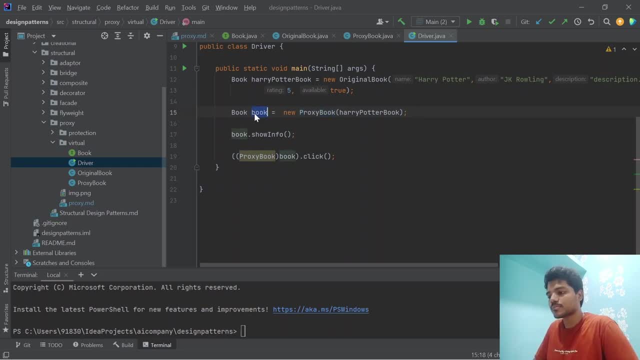 So I am proxying this book. So now this is the proxy book. You can even more clear, like, let's say, you can mention proxy book, So proxy book dot show info. you're just showing only proxy info Whenever someone tries to show the code. 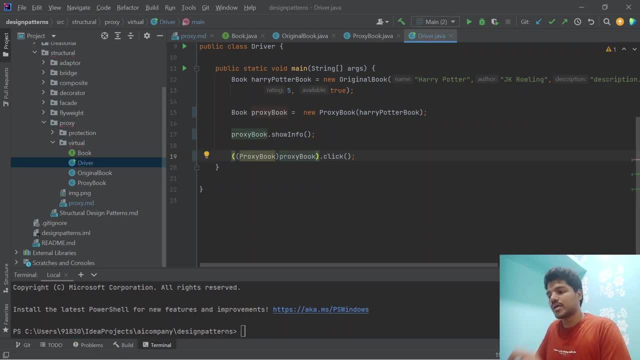 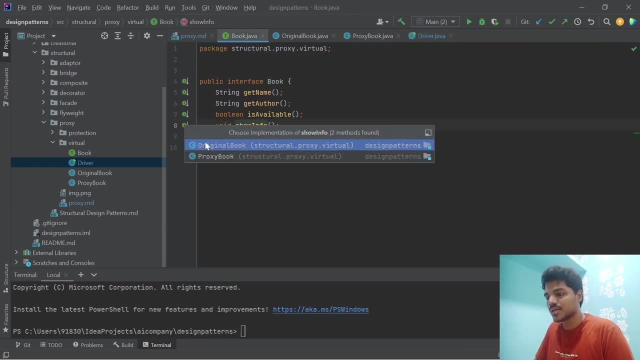 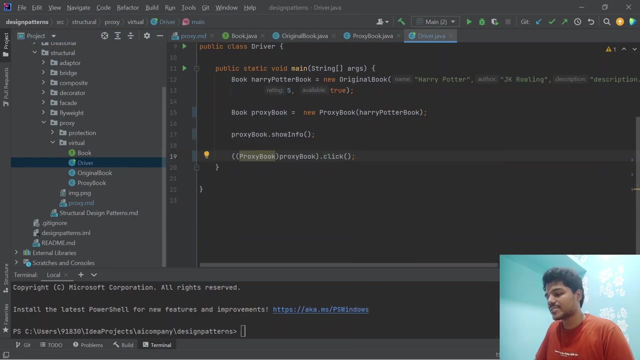 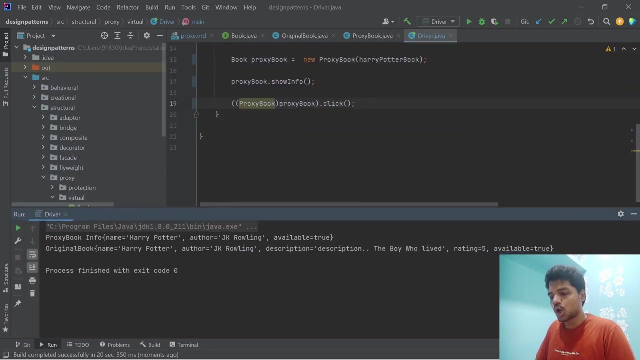 Okay, complete book. you are basically clicking on the proxy book, right, it will display the complete information, like complete book information. so this this click basically calls the original original object: uh, show info which has a complete two string information. let's say, let's uh, right, let's run the program, you'll understand even more better. so if you see right so proxy book. 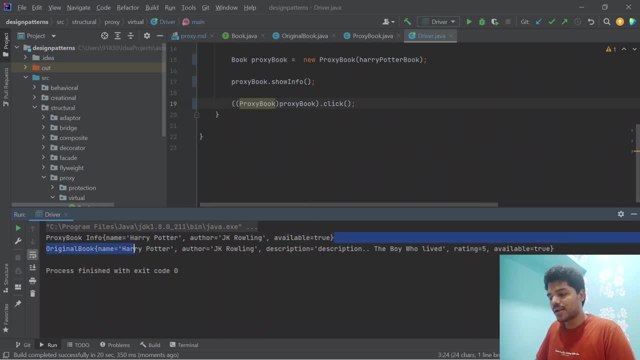 info is basically only harry potter, jk rowling and available is true, but if someone is trying to click the book, we are showing the complete original book, which has like a description rating everything. so that is a simple example of difference between proxy book and proxy uh and. 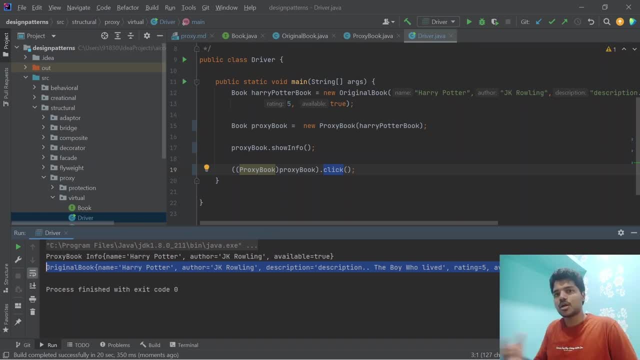 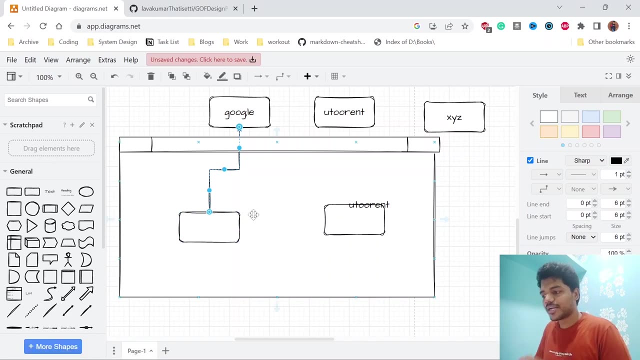 like in a virtual proxy difference between the uh light object and also original object like heavy object. now let's discuss about what is protection proxy. so i have already showed you like what is production proxy through diagram red, which means we are restricting, which means we have some list: is there in an organization we 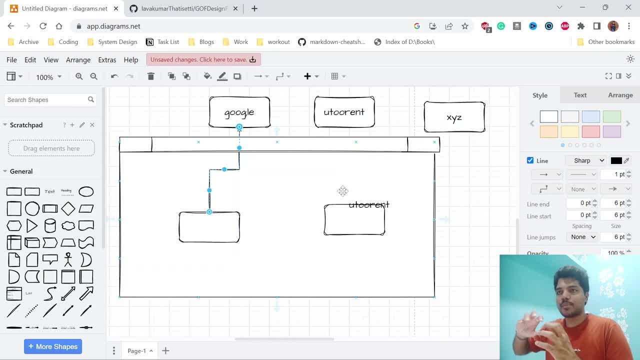 are basically uh, whatever real internet, whatever request we are passing to real internet, we are basically uh proxying that. we are basically uh proxying that one, the complete real internet, and in the proxy internet, uh, we are checking right, so these uh urls are not presented. we. 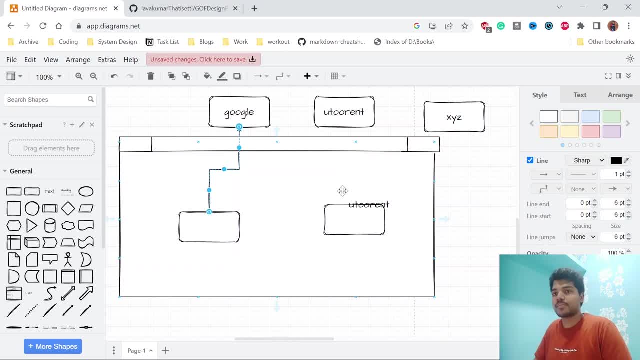 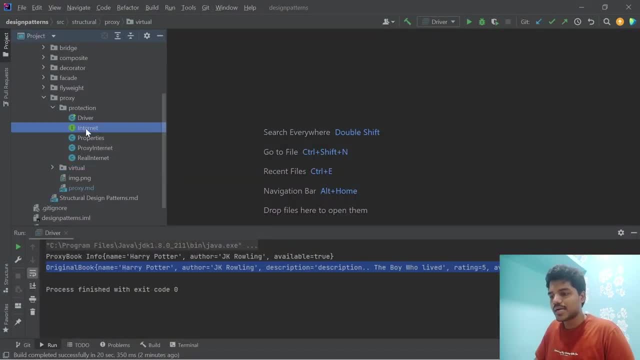 will just pass to the real internet. otherwise we will straight away reject the particular request to forbid, like 403, forbidden or night, or depending upon the custom error configuration. so let's see, we have an internet, is there, uh? which will basically what internet will basically do? it will connect it to the particular url, whatever it provides. so internet basically implements two. 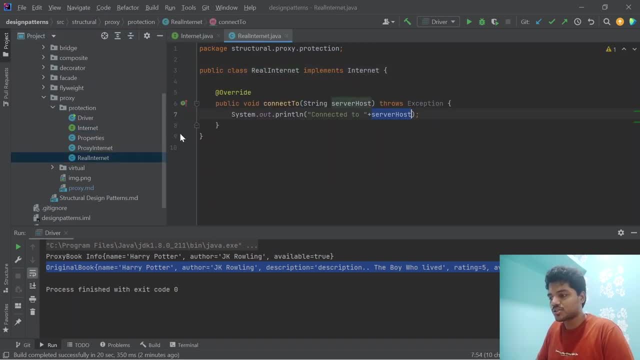 things. one is like real internet, which is basically connecting to the service host. one is like proxy internet. here, if you see, i have properties are there. so i'm basically restricting if someone tries to access the tamil rockers torrent websites, xyz websites. so these are basically malicious. 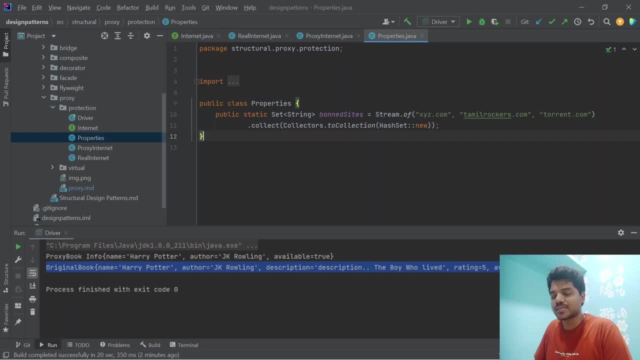 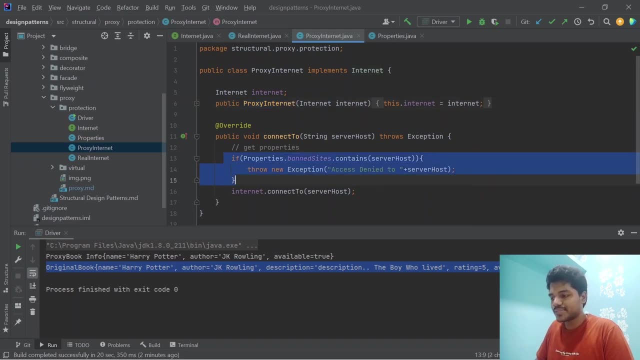 content websites i need to block, uh, if someone tries to access from my network. so basically, uh, so in my proxy internet i'm basically proxying the internet object. so i am checking first if band sets are present. if it is present, i was throwing access denied. if it is not, i was calling the real. 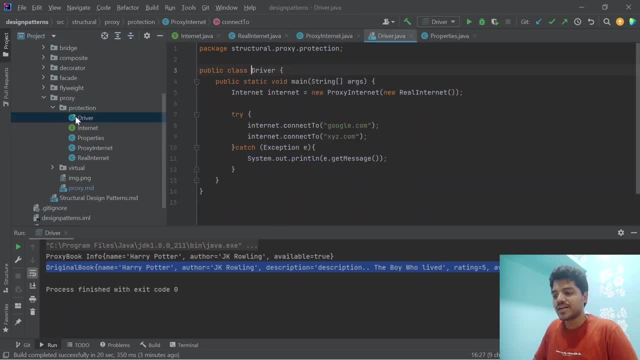 internet object to connect it to the actual internet. so if you see the driver program right, initially i have a real internet object. i was proxying this real internet object with the proxy internet. now i have created the proxy internet object. uh, when i was trying to connect to the 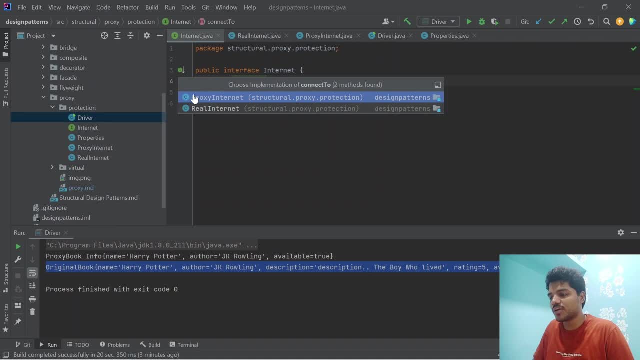 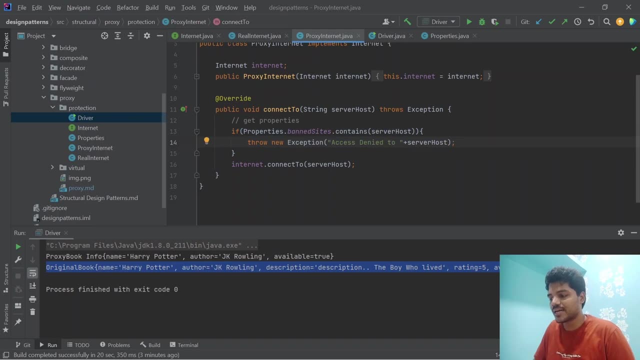 google. it will first basically checks the. it will. it will first basically check, uh, whether these, whether whatever is there in the band sites or not. if it is there, it will be basically access in it. otherwise it will be connected to the real internet here. so, uh, let's execute the program you. 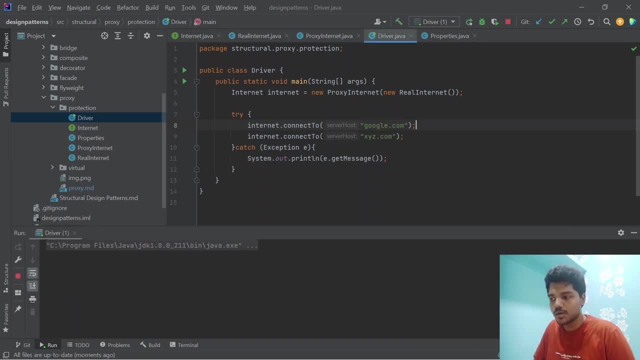 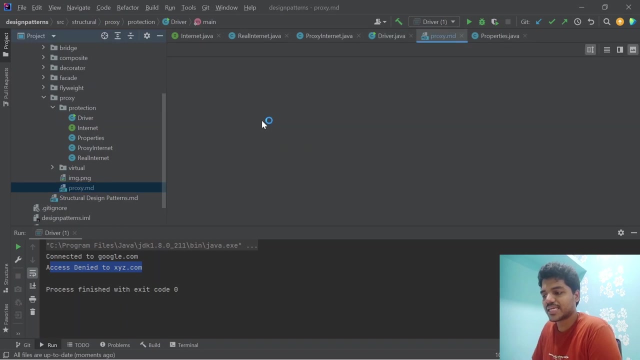 will better understand. so first one. according to this program, first one should be allowed and second one should be rejected. see: connected to the googlecom successfully happened. so instead access denied to xyzcom. so this is exactly what production proxies. so proxy design pattern is like very easy design pattern and also many people don't know about this. so let's go to the proxies. 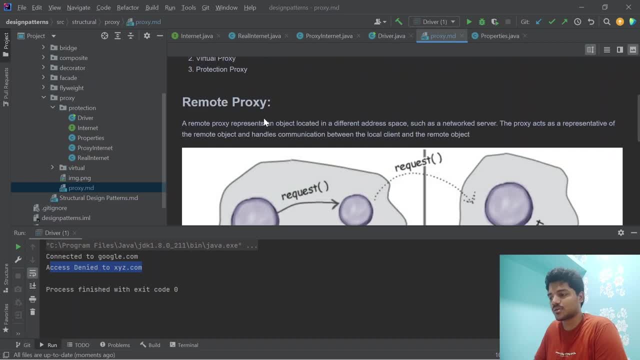 design pattern and also many people don't know about this, so let's go to the proxies design pattern. and also many will use this proxy design pattern in companies or like in organizations. so let's once go through this video again if you didn't understand, once go. 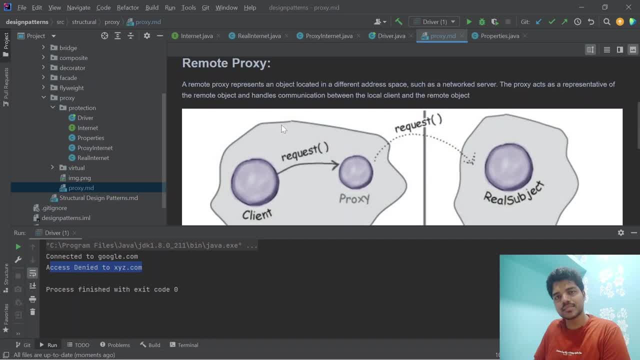 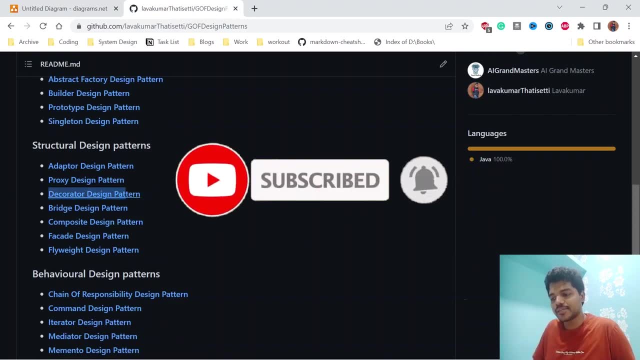 through this what you call like this MD file, you will understand even more better. so I think that's it for today's tutorial. in the next video I will explain decorator design pattern, which is basically similar to proxy, but there is quite changes of proxy design pattern. so we'll soon meet with the